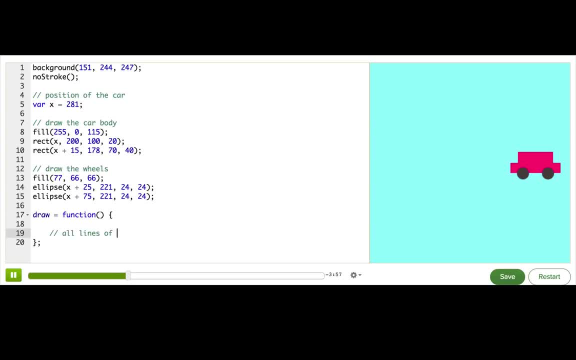 times a second. So all lines of code inside here will be run repeatedly, Everything that's not inside this function. so all of this will only get run once when the program first loads. So we want to get our car code in the inside of this function. I'm going to select all of it and cut it, paste it in. 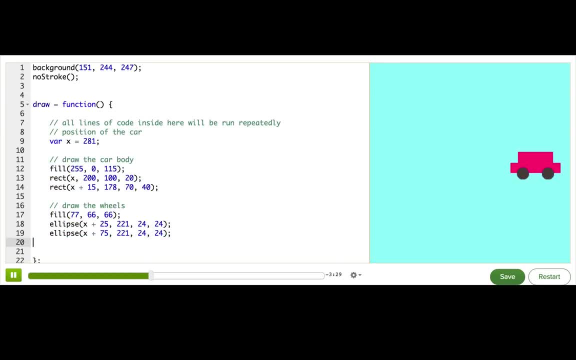 here, Then I'm going to indent it so that it really looks like it's inside the function in between these curly braces here. All right, now everything looks the same as it was before. Well, it looks the same. It actually isn't the same. We are. 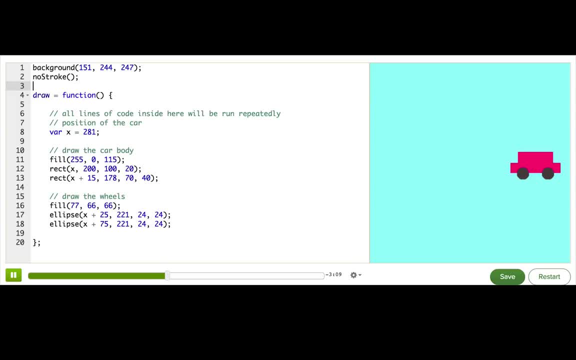 now actually having our car drawing drawn over and over many times a second, But it looks the same because it's always getting drawn in the same spot, right? Because x is 281 and that x gets fed into this rectum, these ellipses and the x. 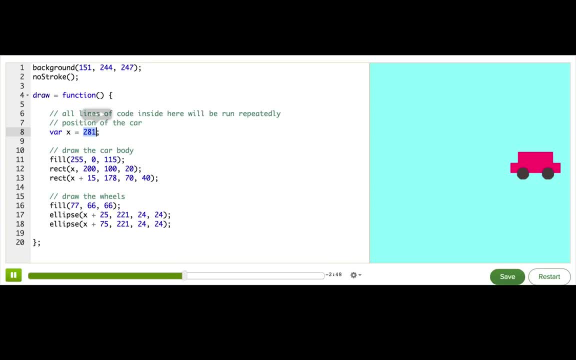 stays 281 every single time, So that car is not going to move, It's just going to stay there. We want the car to be in a new spot every time. Conceptually, we want to be able to tell the program: let's start the car's x position at 10 and then add 1 to that position in every. 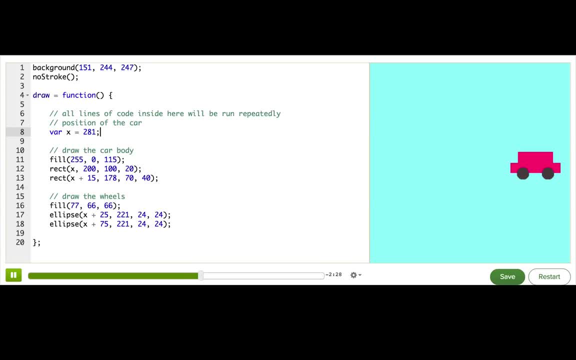 drawing of the animation. To do that, I'm going to move the x variable outside of the draw function up here, set it back to 10.. Now, since this is outside the draw function, this line of code will get run once at the beginning of the program. 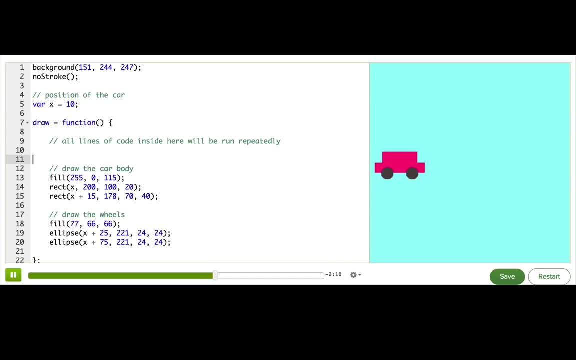 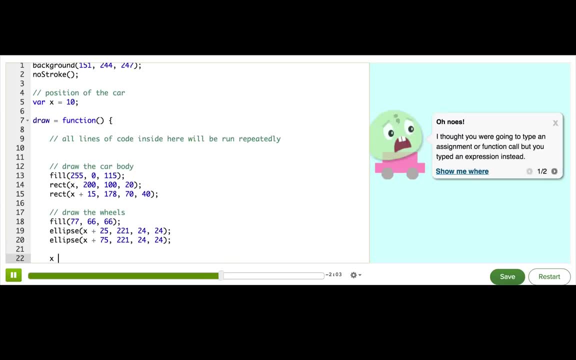 setting x to 10.. Now, inside draw, at the very end, I'll add a line of code to add 1 to that variable. So x equals x plus 1.. Ha, ha, It's moving. Alright, it's a little smeary, so it looks more like paint than a car. The reason: 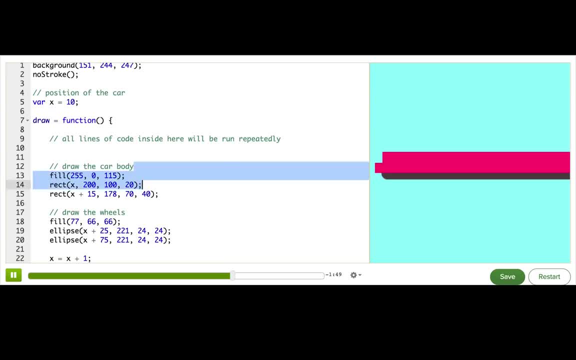 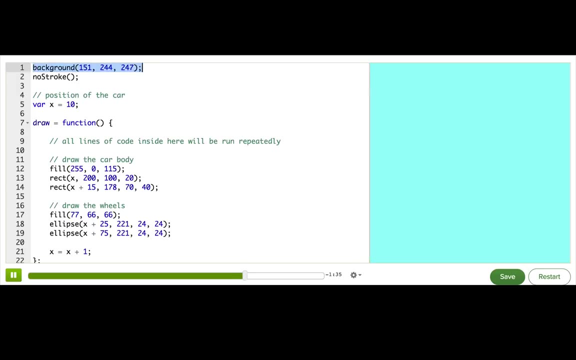 it's smearing is because we're telling the program to redraw the car each time, but its redrawing it on top of the car from before because it's still there. If we want the program to to erase the car from before, then what we can do is take the background call.